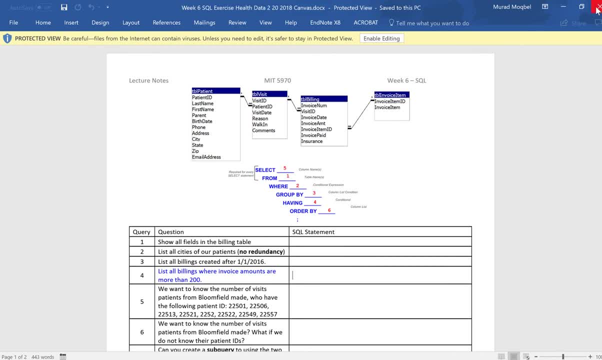 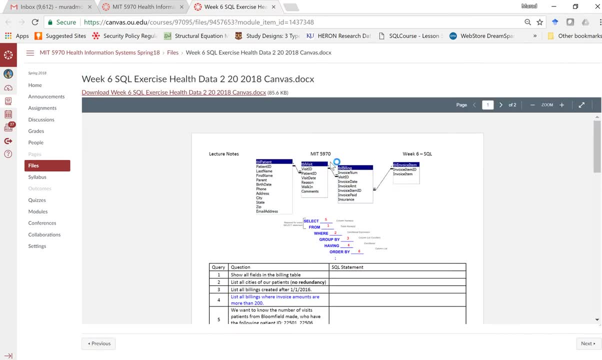 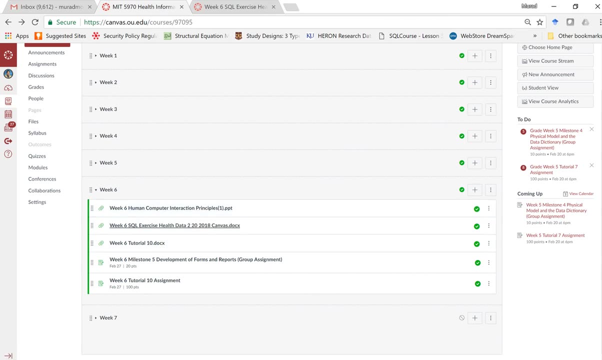 Alright, so that's for this SQL, Regarding the SQL Exercise, but the other one is, so now the next. the other thing is that we want to go over the Human Computer Interaction, and I want to briefly go over some of the points because this is part of the reading. 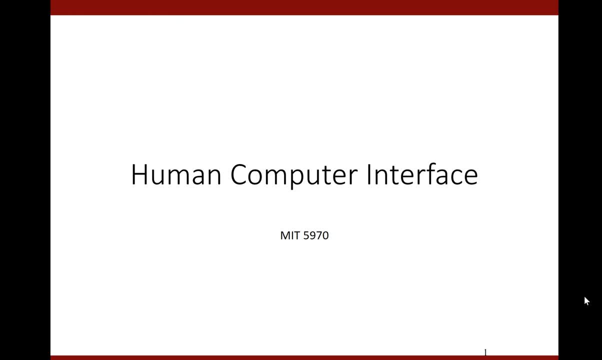 So I will let you read this. So I will let you read those slides, because they have very valuable information that will help you. So I'll tell you some of the points that will help you take a look at this process. So let's go ahead and start. 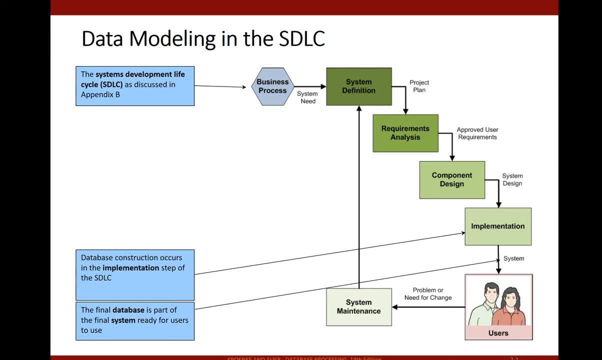 So let's go on. so so far, this is what we have been doing so far and we have been going through the system development life cycle. And actually yesterday I went along with the dean and we met with the dean of the School Health Professions at the OU Medical Center and they have been 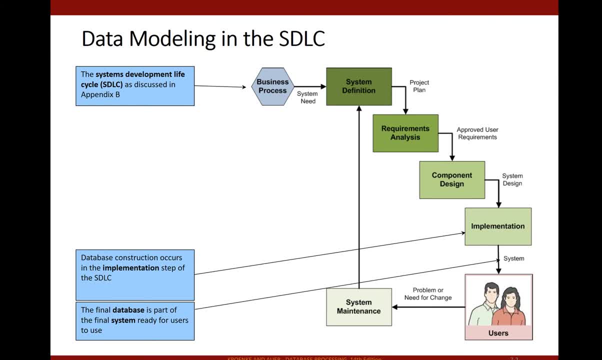 Been working with the dean and we met with the dean of the School Health Professions at the OU Medical Center and they have been- And they have been actually appreciating that we are offering this class because it turns out that they don't have an electronic health records yet at the School of. 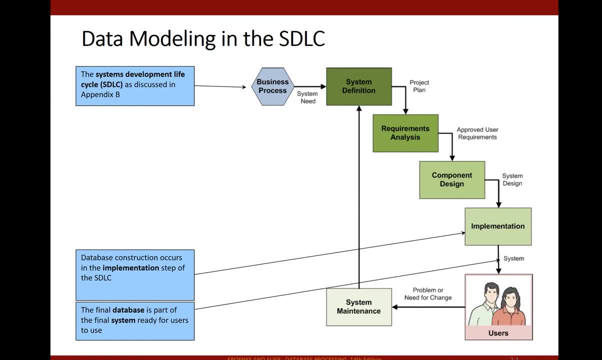 Health Professions and they are still using the paper-based system that we talked about for this particular example, for this facility. so they are looking for people with this skill that can help them transform from paper-based into a an electronic health record system, and so this is kind of emphasizes the 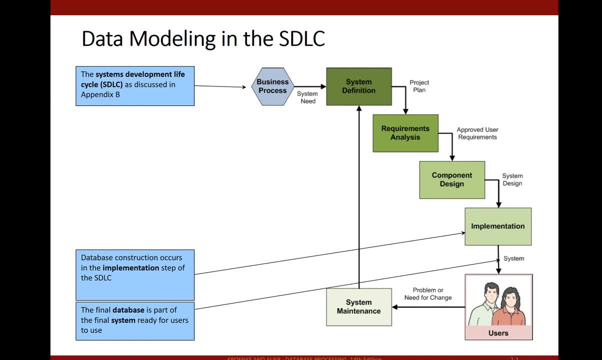 benefit of this class and I hope that you have been getting a lot of valuable information and valuable skills throughout this class in terms of project management, which was in the first phase of the system development lifecycle, and then with the end-user requirements that we talked about earlier. that's a huge benefit and I'll see you guys in. 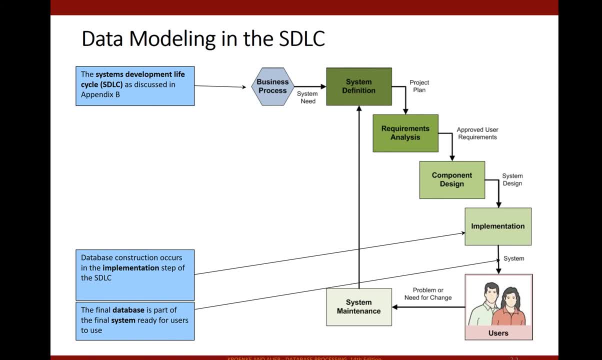 was another important skill that you can actually put it in your resume. so project management is one of the skills that you can put it there. another skill is end-user requirements. this is where system analysts, or business analysts, most of the jobs actually are based. so requirement analysis- you, you did that. 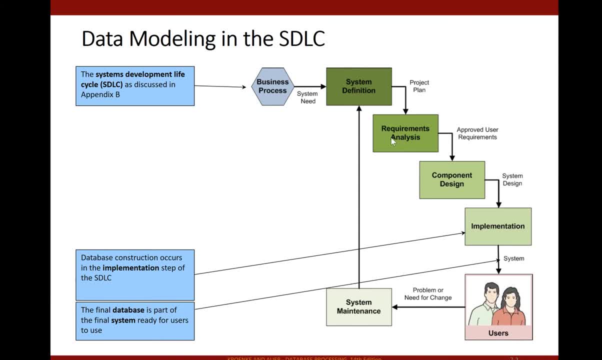 through interviewing the end-user and examining existing documentations of the client. and then we we moved on to the component design and we said there were three: component design and the conceptual model, where we just developed or built those entities which are based basically themes, and every theme has. 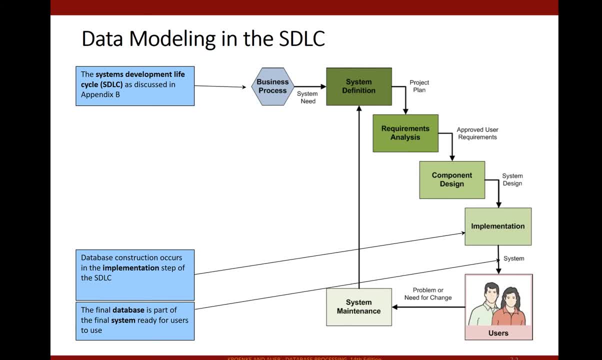 characteristics that we want to collect about it, and those characteristics are basically the attributes for each entity. and then, in the conceptual model, we connected or we created those entities, and we connected them along with the cardinalities, the one-to-many, one-to-one or many-to-many, and then we, we went on to. 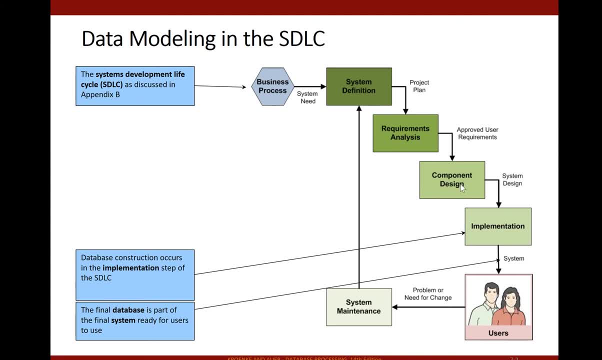 the next design model, which is so we transformed or we went from the conceptual model into the logical model while we were in component design stage. so the logical model is the model we created and we created those entities. so we where we decided where to put the foreign key and we had also rules of 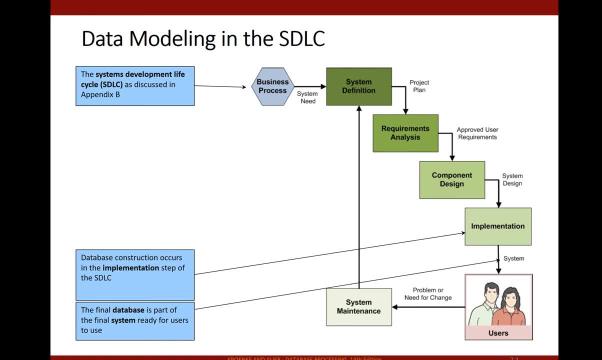 thumb where to put the foreign key when we have a 1 to 1 maximum cardinality and 0 to 0 or 0 to 1 minimum cardinality. so we all, we covered that already about the logical model, and then the third model was the physical model. will you where? 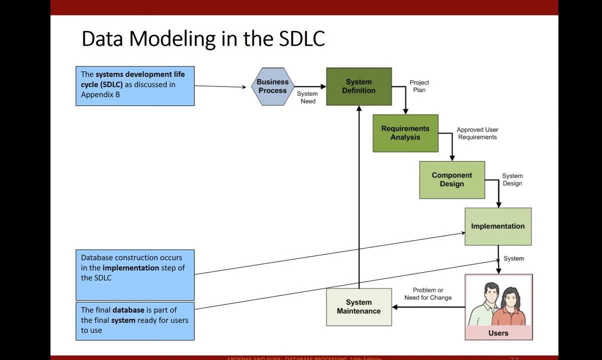 you transform the logical model that you had built and you transform that into an actual database and actual tables and you connected those tables and that's what you actually submitted, or you, you submit it today. so you created those tables based on the interrelationship diagram that you designed and you built. 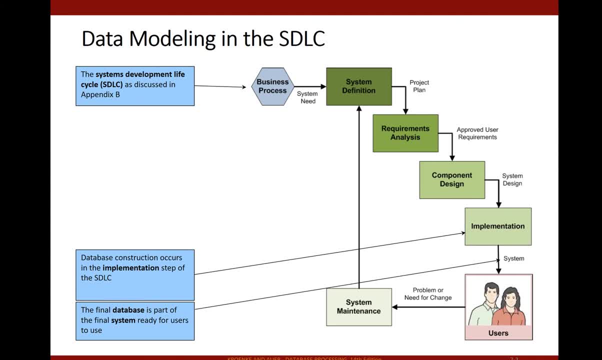 from scratch, and now you will see the fruits of your hard work that you have done so far and then, based on that, we will be able to create forms and queries and reports. so now we moved. actually, we are kind of in between the component design, which is 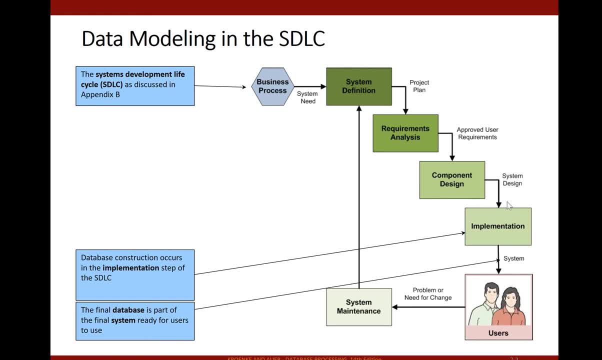 the physical model and we already kind of started with the implementation, because we already built that, the tables. so now the implementation will be completed after we create the, the forms and reports. and so let's, in order to create the forms and reports, we need to understand the. 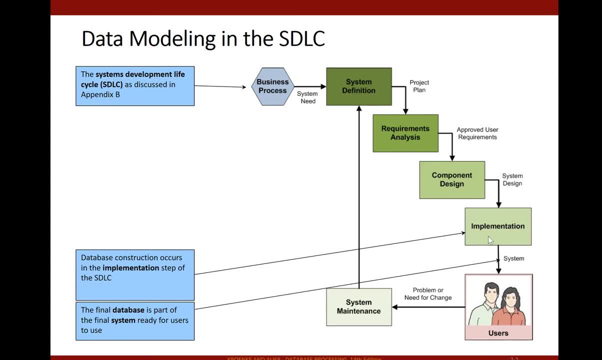 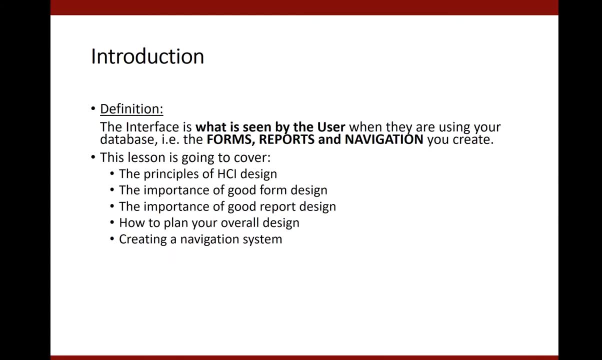 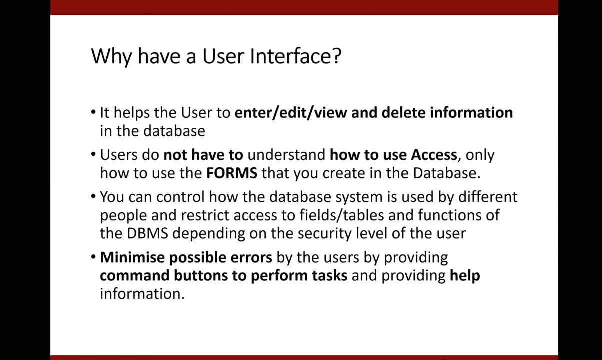 basic and the foundational principles of human computer interface or interactions. so I will let you read some of those. so I will skip some of those slides because I will let you read them, and I will just go on and highlight some of the the points why user interface is important, because it enables the end. 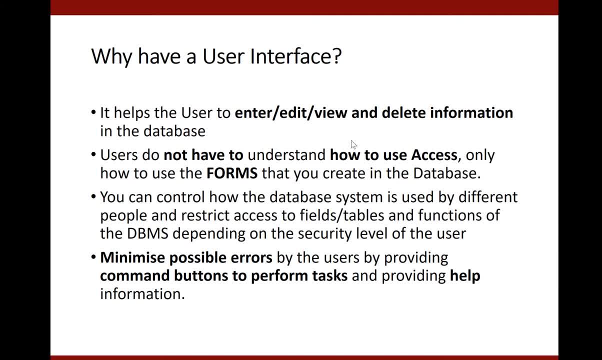 user to edit, enter and view and delete information, So the end user doesn't have to learn or to be able to create a database in Access, but they need to be able to use those forms and reports that you created for them. That's kind of the main, the most important aspect of the 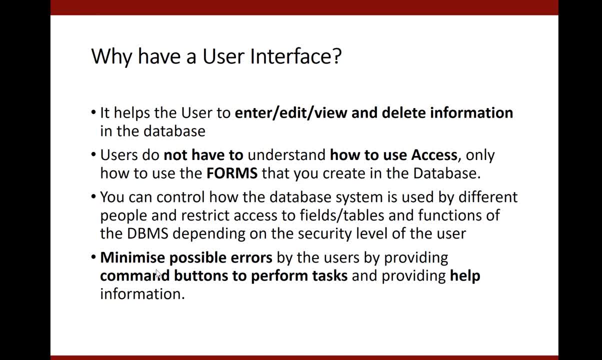 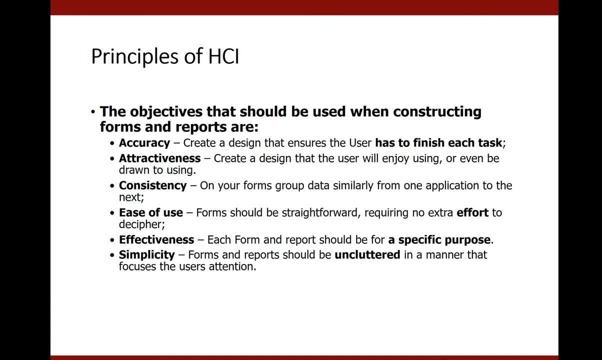 project that you, or the system that you develop, and also another important aspect of the project you developed, is minimizing possible errors, and we have- we went through the normalization process and we have used a lot of techniques to minimize errors. So what are the principles or the objectives of? 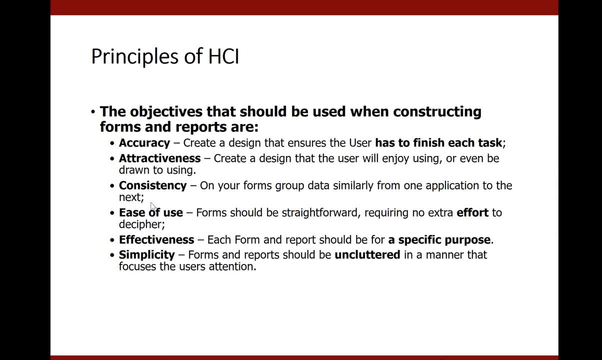 constructing forms of reports is accuracy, So the principles of a human computer interaction or interface, is accuracy, meaning that the end-user has to finish each task accurately and successfully. And the second one is attractiveness. So, as well as finishing each task accurately and successfully, and the second one is attractiveness, So as 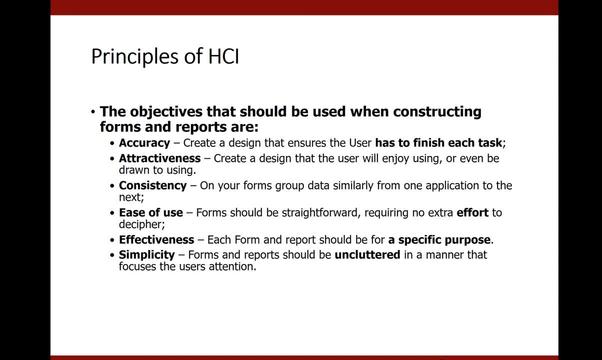 don't forget, we have the principles and principles of a human computer and Oh So, as well as finishing each task accurately and successfully. And the second one is: we all know that attractiveness is is very important, and actually I just read recently about the the role of attractiveness in terms of technology. 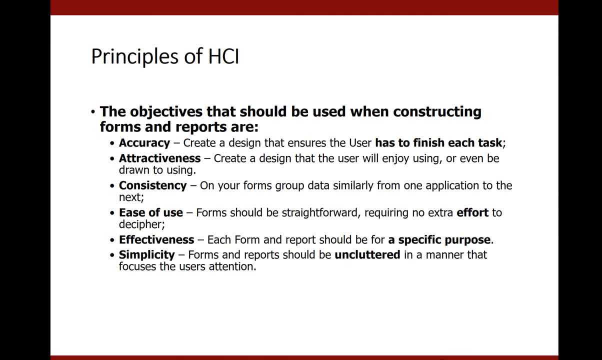 addiction and it turned out that addiction of information technologies, such as phone addiction, is resulted from the beauty or the beautiful design of the phone, the beautiful colors, the beautiful icons that we see and we turn. we tend to be addicted to checking our phones because of that beautiful color. 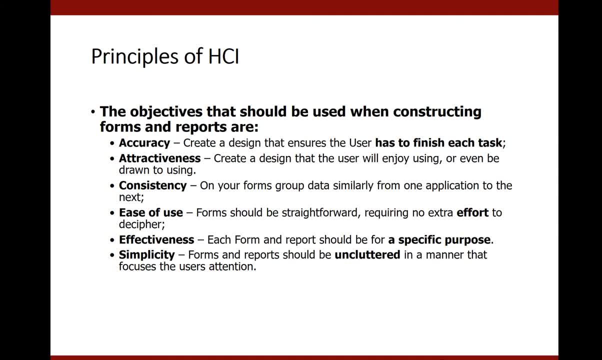 and beautiful design that we see all the time. so, again, it is very important and it is helpful if we can create that addiction for a very beneficial tool such as the database that you, or the system that you are- electronic health records that you are developing, for that, for the 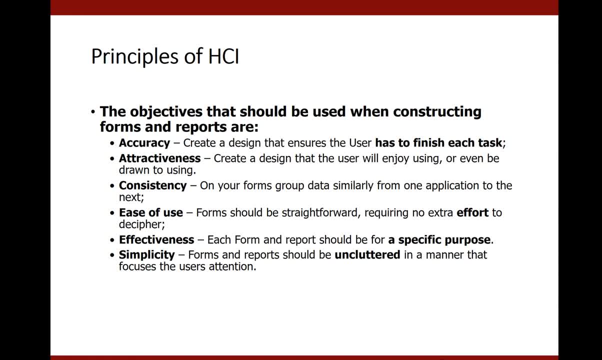 nervous system. So I think that's the most important thing that we can do in this, in this scenario. so attractiveness: it needs to be beautiful for the end user to use it. and then consistency: all the forms and reports they need to use the same colors, kind of the same themes, the same feel that you have for them. so it needs to be. 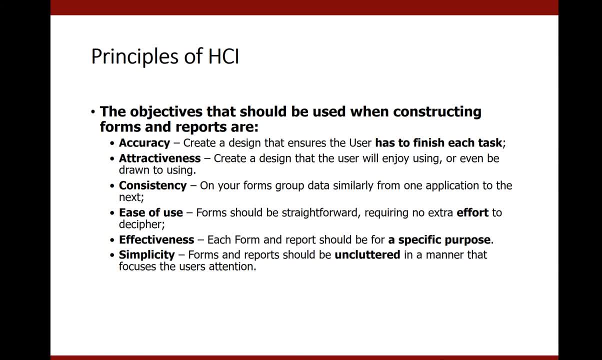 consistent: when you are using navigation buttons, they need to be in the same place in all forms, and and if you want to use them in reports also, they need to be in the same location and using the same sizes, and so on. and then the ease of use. ease of use here what we mean, not only that the system needs to be easy to. 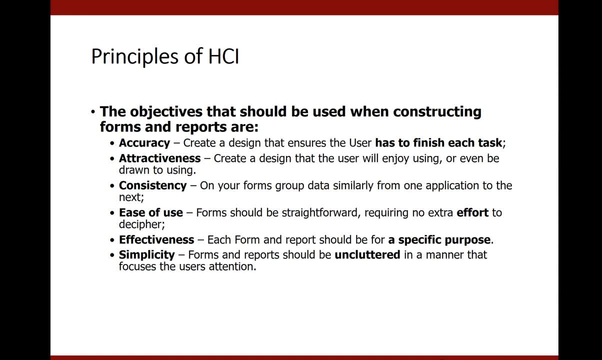 use, but also it needs to not require cognitive efforts from the end user. the end user doesn't doesn't have to remember anything while they are using the system, so try to make it as simple as as easy as possible for the end user not to have to learn something every time they use the system. 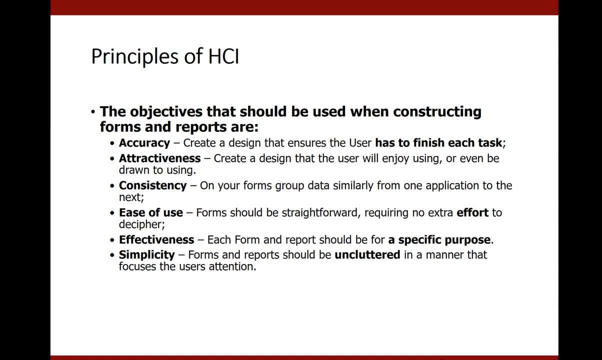 and they don't need to use their cognitive efforts and remember things. so that's what we mean here by ease of use. Effectiveness means that the end user needs to be able to complete the tasks with perfection, and for that specific purpose and simplicity, here we. what do? 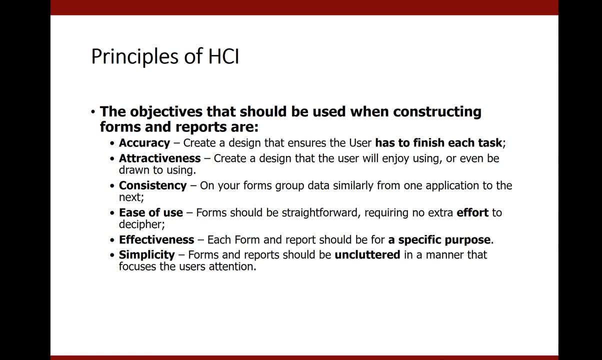 we mean by simplicity is that the form or the report needs to be in a simple matter. you don't have to use some of those colors that are annoying or or just distracting. it has to be simple. you can use black and white, for example, but you can use other colors. that's not that what I want to mean. what I want to say. 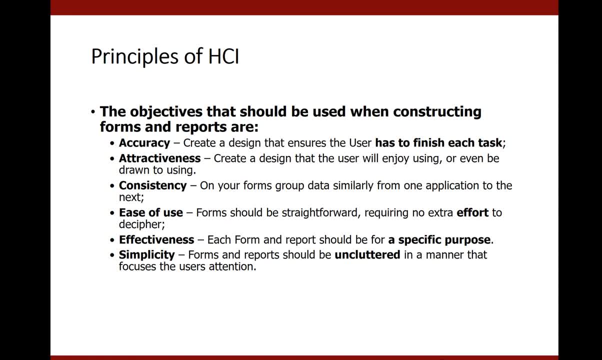 here. but simplicity is that you don't clutter the form with all kinds of things. it needs to be simple if you use, let's say, black and white colors and make use of the spaces, make sure that there is blank spaces and and empty spaces here and there for us, for the end users, to breathe, rather than overwhelm. 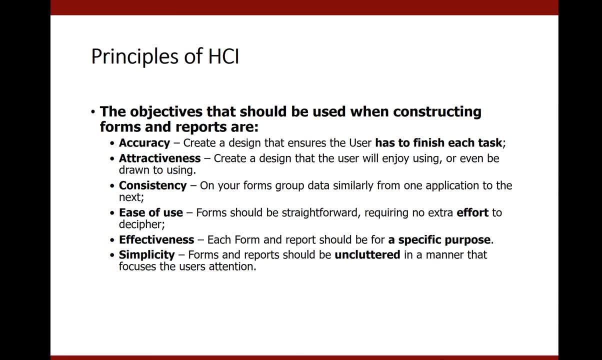 them with text all over so you can minimize, for example, you can use the tipping or you can use, for example, help buttons. instead of putting so much content in the form, you can put it in a help button where, if they need more information about a certain certain button or a certain field, they can click. 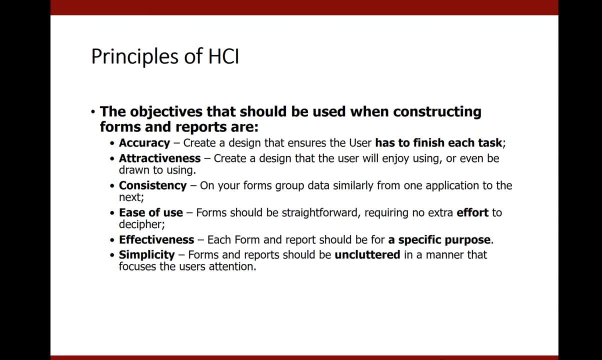 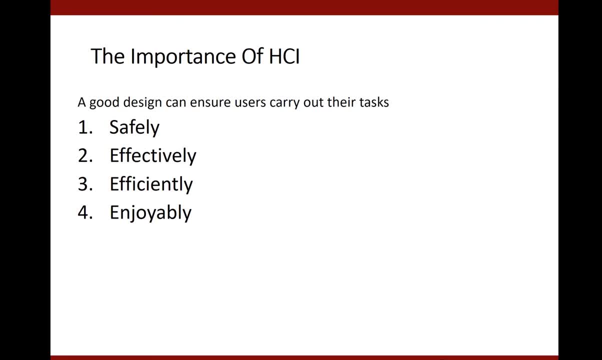 on that help button and then a new form opens up that has more 燽 details about it. So that's what we mean here by simplicity: Don't overwhelm the end user with content. So a human-computer interaction or interface is very important so that the end user can complete their tasks safely. 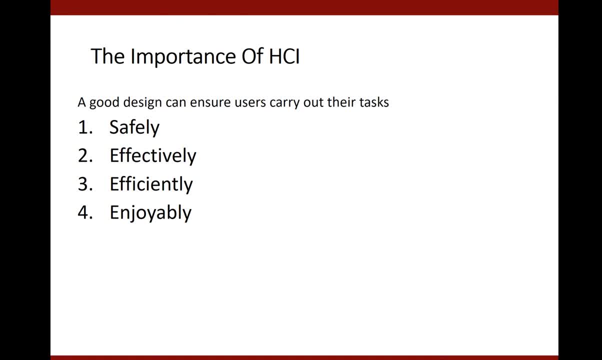 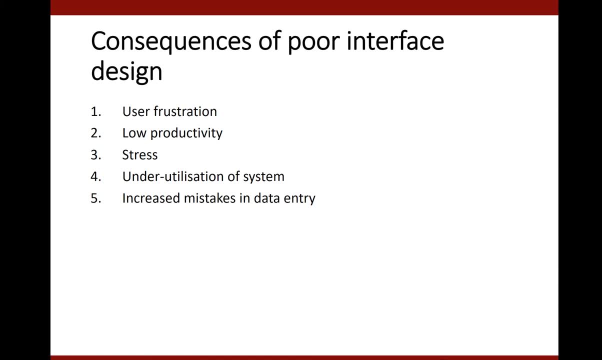 effectively, efficiently and enjoyably. Basically, this summarizes what I just mentioned earlier. So the end user needs to be able to finish their tasks with high quality user interface, Because if they don't have high quality user interface, then it will lead to user frustration and low productivity. Because 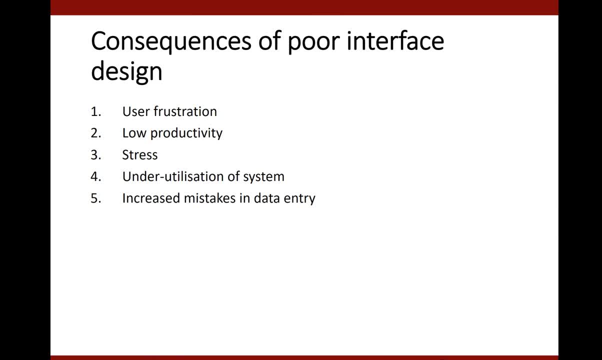 if you are using a form that is not, let's say, saving the content, every time you will assume that it is saving it, but it's not saving it. then you will have to go back and redo it, So it lowers productivity in that sense and increases 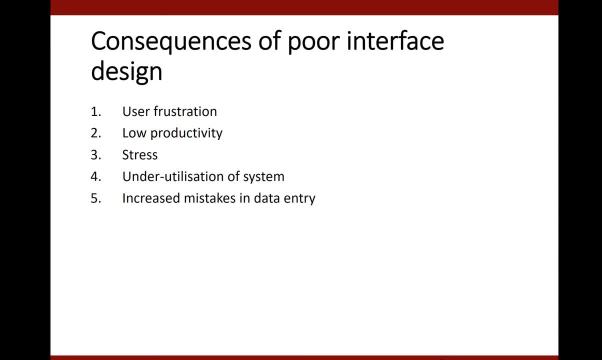 stress. If you are trying to get it to do something and it doesn't and keeps giving you error message because of that poor interface design, then it increases the stress. And, as I said, nurses, they are already stressed because of their job and we don't want to over stress them even more with the system. 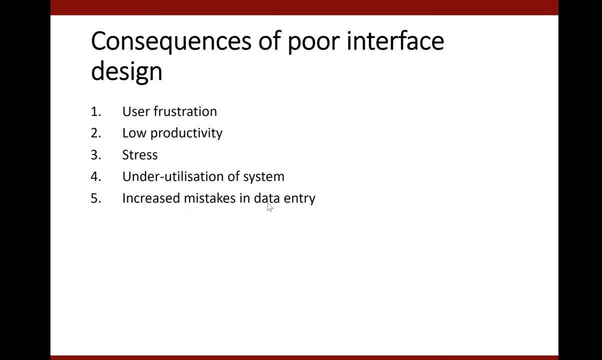 that we develop for them. And then they're under utilization of the system, because if we have poor design, then the system will be underutilized. So we need to keep it simple and the user interface needs to be high quality so they can be utilized well. Increased mistakes in data entry. So we will try to. 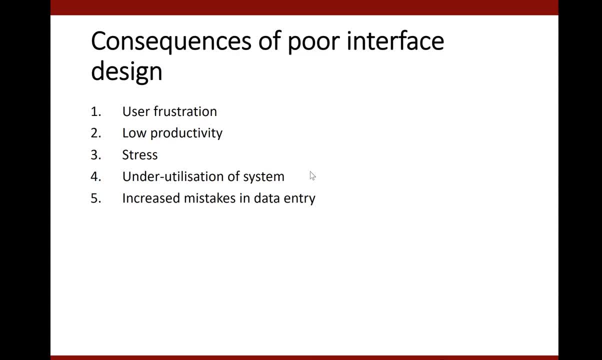 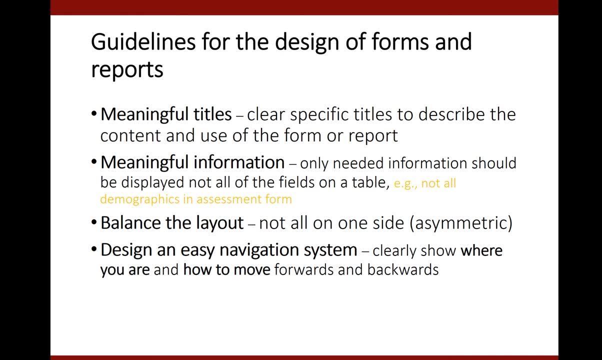 avoid all of those poor or negative aspects of design. So here are some of the guidelines of the design of the forms and reports that I want to emphasize. First, meaningful titles For every form, every title they need to have. every form, every report need to have meaningful titles. So we have learned how. 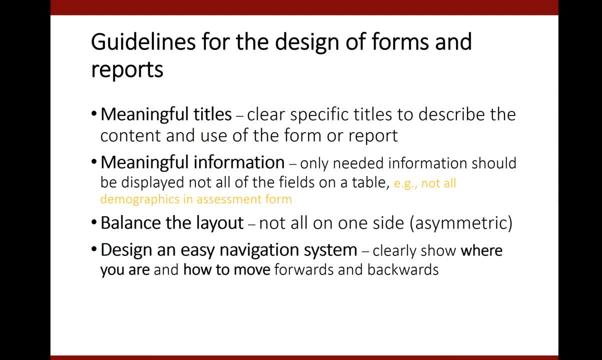 to create titles so far and those styles. they need to be meaningful. For example, let's say that two main forms, that you will need at least two main forms in your database or in user application that you are creating. one form needs to be called resident, demographics or resident, and that resident form 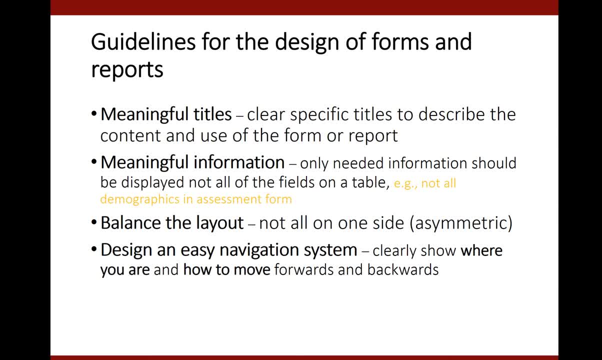 Invent. rents can be a main form with several sub forms, but that form has to have all the components of the resident: Their names, their gender, their addresses, their phone numbers and phone types, and then also their diagnosis. So that's one form, and then the other form is the assessment form. 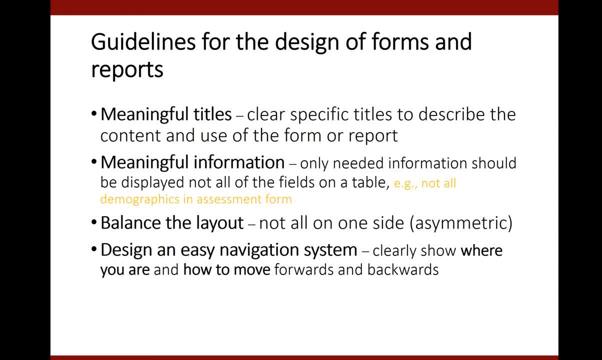 and the assessment form needs to replicate the paper-based form that you have been given in the request for proposal and those documentations that you were given. So those are the two main forms that needs to be included in your system, as well as for the reports, You have four reports that were requested and they have more details about what they really 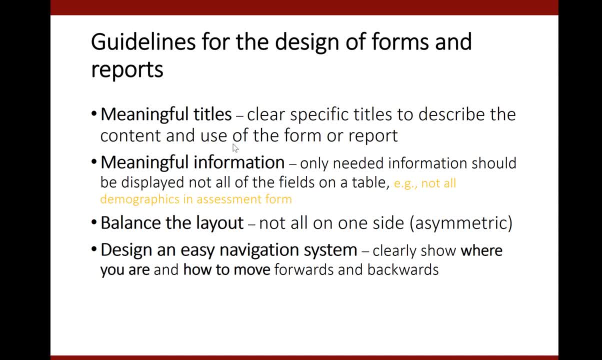 want. so make sure that you have meaningful titles for those. So for the assessment form you can call it assessment form and the other one you can call it resident form. But by having those two you, it is kind of comprehensive. Those titles are comprehensive. they kind of indicate what we really want, to, what what we are collecting from for them. 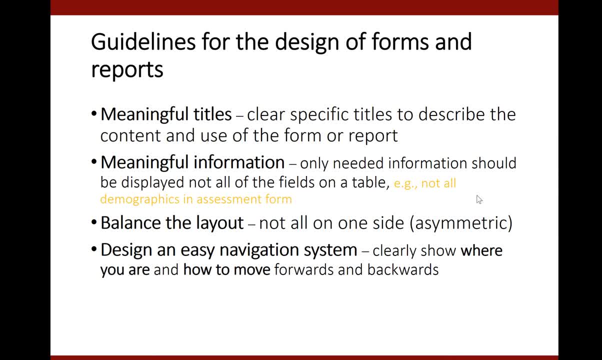 And then meaningful information. So what do we mean here by meaningful information? is that in the assessment we don't need to include, let's say, fields that don't add any value to the end user. For example, in the assessment table we have a primary key, that is a surrogate key. When we say the surrogate key is a system generated primary. 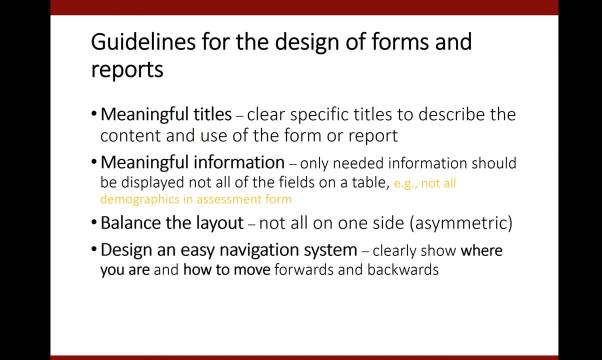 key that doesn't have any meaning by itself. For example, it goes from one all the way to infinity. In that case we don't want to show that It is not meaningful information, so we don't want to show it. Or here, not all demographics in the assessment form need to be shown in the assessment. 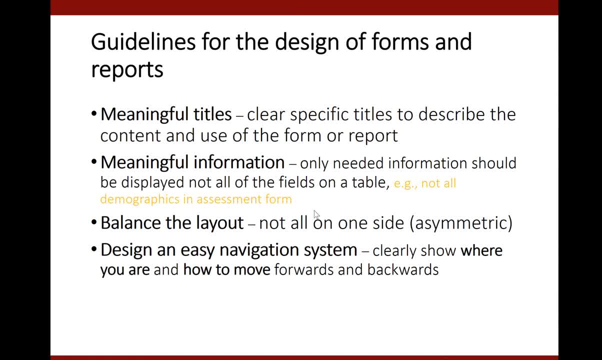 form, For example, we just need their- maybe- names and verify maybe their date of birth, but just whatever the original paper-based form was showing. So that's what we want to show And then balance the layout. So another guideline or another important feature of user interface is: 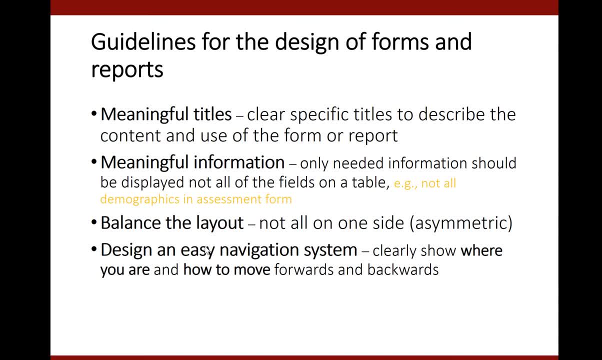 the balance layout. This is what we mean here by symmetry. If you have taken an art appreciation course, you might have gone through the symmetry concept, where you want to make sure that the user interface or the picture or the image that you are working with is balanced from the right side. 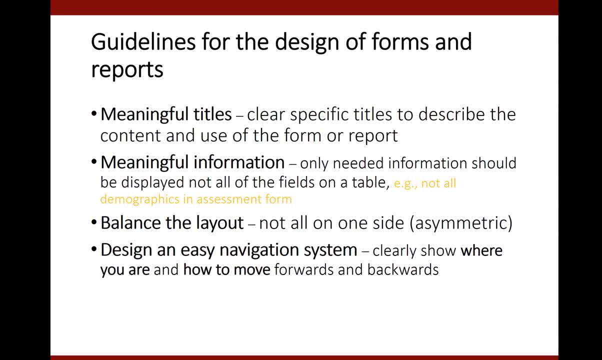 to the left side. So we need to be making sure that the interface is symmetric And then design an easy navigation system. So it's very important that the end user knows where they are and how to go back and forth. For example, let's say that as soon as I open the system, I need to go to a main menu And then the 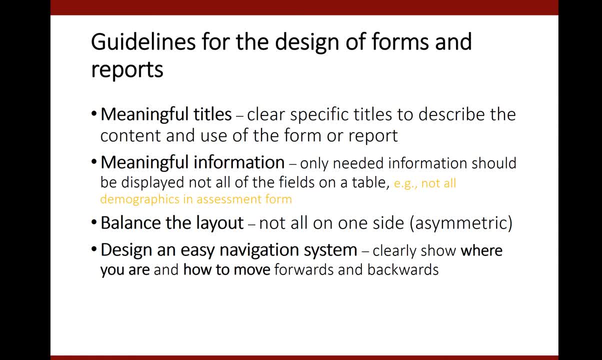 main menu should navigate, or should I should be able to navigate as an end user, from the main menu to other forms, Let's say to the resident form. When I am in the resident form, I need to be able to navigate to go back to the main menu or to proceed to go into the assessment form. So I need 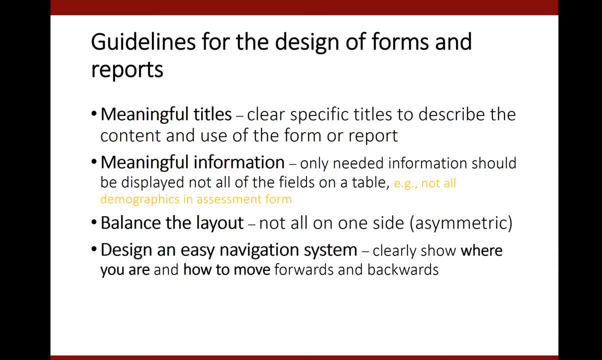 to be able to know where I am and how to go back, Because some bad design that I have noticed in some systems that it takes you to a one page and then you don't know how, especially if you PeopleSoft when you are there, then you can't go back or you have to close it and go on. 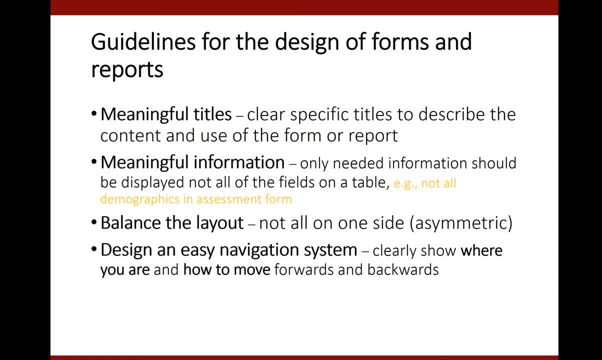 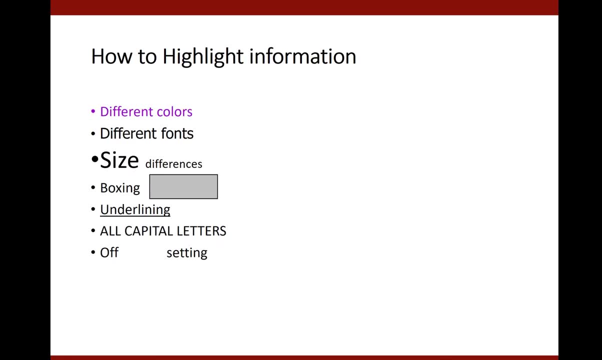 and log in and in order to go and visit another page. So it is not friendly in that case. So for us, we will need- we will try to avoid that- Making sure that the navigation system is clearly stated and inputted. And then how can we highlight some? 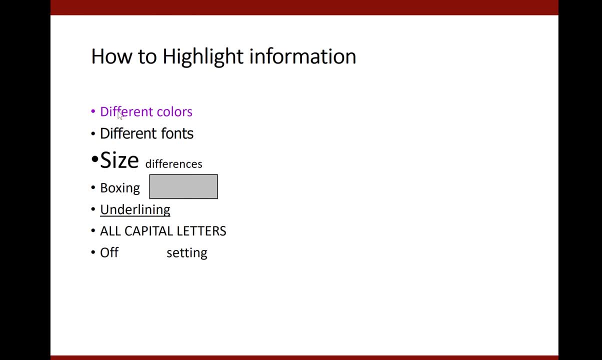 information. As you can see here, the color played a very big difference here because we are using purple color. So color is one way that if we want to highlight some information- And in your case you remember we said that the end user emphasized, or they wanted us to use color for conditional formatting, for example, for 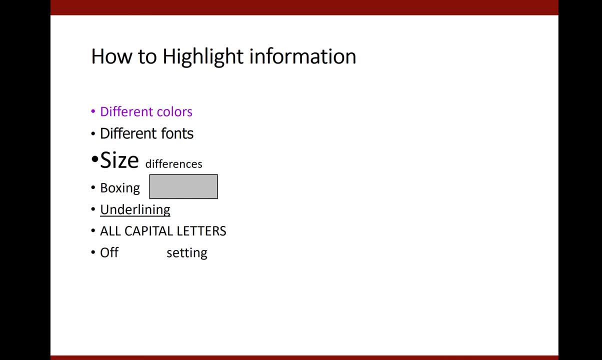 red for high risk And yellow for medium to low risk, and no risk is in green. So that kind of highlights some information for us And then different fonts can also highlight information And the size also shows the difference and importance of information. 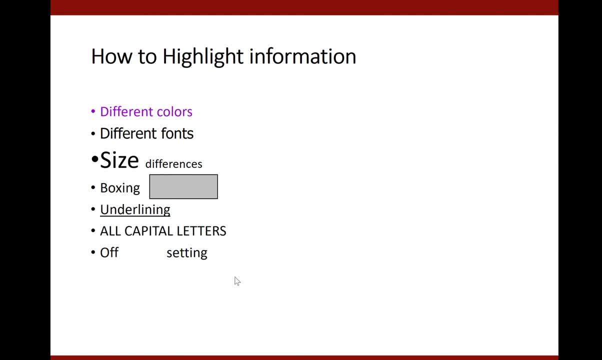 Boxing, also underlying using all capital letters. But I would. I would be conservative in using all cap letters because many people understand All cap letters as shouting or yelling at someone. So we don't want to yell at anybody, So let's avoid that. all capital. 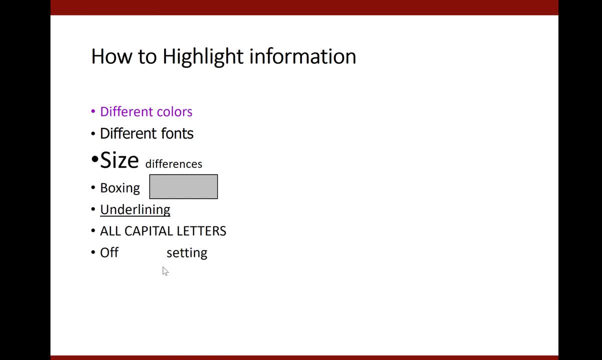 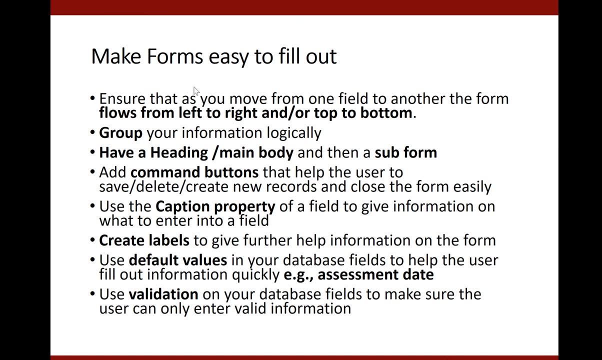 letters And then of setting here spaces, kind of also shows that there is an importance, So. so we need to make sure that the forms are easy to fill out. So here, what we mean here by it, flows some, some forms that we, when we tell them out, they can be. 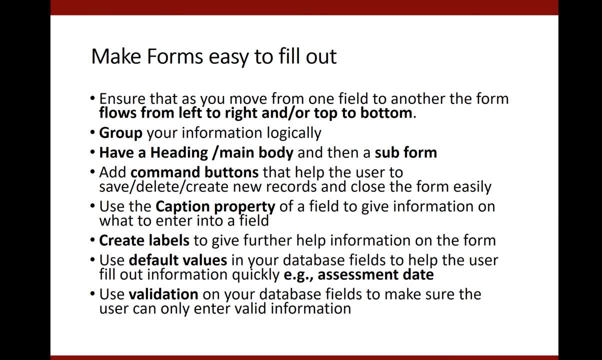 let's say two columns, So one form can be filled out, let's say from top down, and then we go to the next column, top down. So that's kind of just like an N shape to some extent, you can say, or a inverse N shape, but so that's one way, the flow. 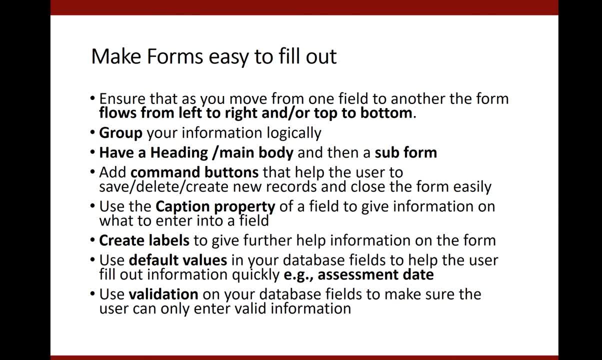 needs to be consistent, To start from top down and then top down, or you can go from left to right and then down, from left to right And then probably three, if you think about it. So the flow from top down and then from top down, and then you can go from left to right and then from the other way. 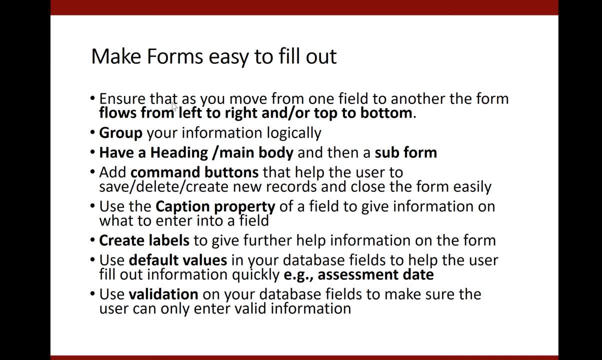 to right. so that's what I mean here by the Z, the Z flow. so you start from left to right and then you go down and then left to right and so on. so it needs to be logical and then grouping also helps. for example, if I am talking about the 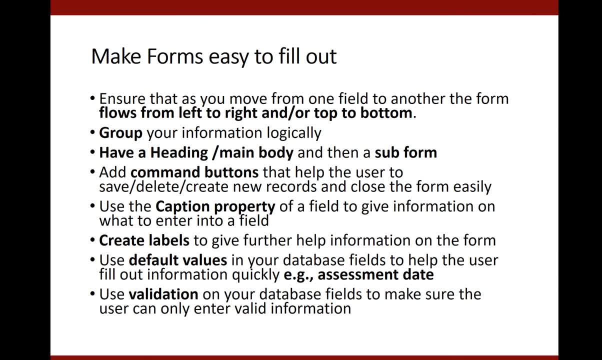 address in the resident form. the address needs to be grouped by itself somewhere in the form and let's say the phone numbers. it should be grouped by itself. diagnosis should be by itself. so that's what we mean here by grouping and so having a heading or main body and sub form. so heading again it helps, kind of. 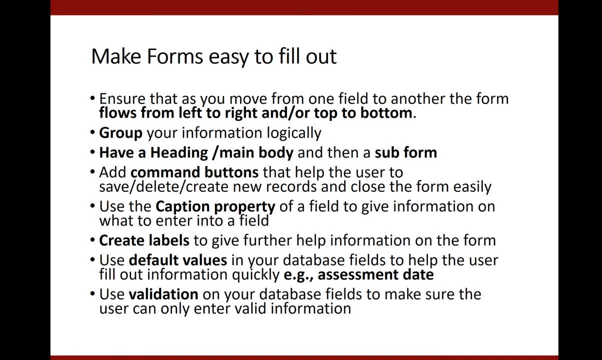 to have a heading for a sub form. for example, if in the resident form you have one form that will be filling out diagnosis, so I need the heading for that diagnosis and you can call it diagnosis, and then I need heading for phone numbers. or I need a heading for address for 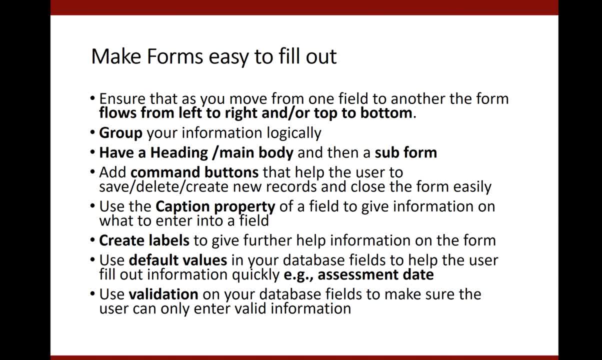 example. so it's very important that we keep this in mind when we are developing the user interface forms so, and we need to add command buttons. so the command buttons here help us kind of to save, maybe move forward, move backward. so command buttons are very important and also command buttons can help us to navigate from. 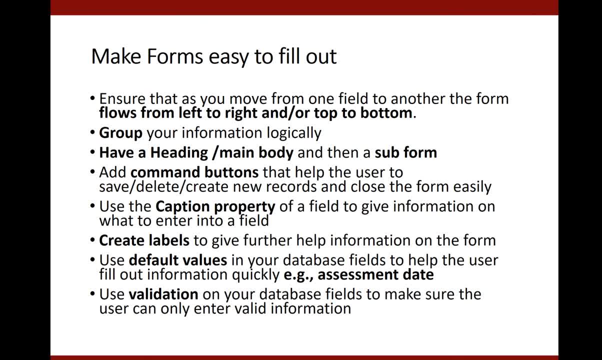 that form to another form, or from that form to the main menu, or from the main menu to some form, to other form, or from the main menu to the main menu, or from other forms or to other reports. so navigation or command buttons are very important, so let's make use out of them. and also you can use close buttons to 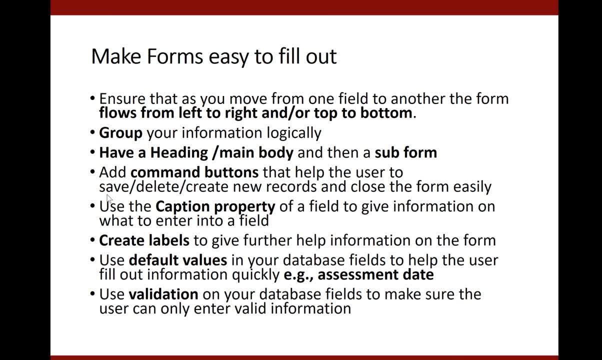 close. I would not use delete, but I will maybe save and close buttons and then navigation, going back home or going back to the main menu, and then I will use caption property. so caption some people, if you have noticed, in some forms they gave you kind of 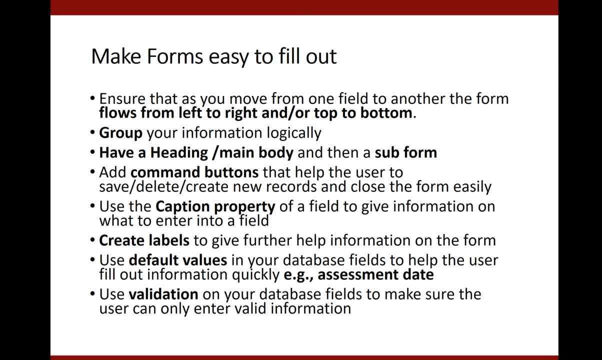 an example how to fill out a date, for example date of birth. so how the date of birth? I will. I will use input mask for it, because I don't want people to open. let's say that- the calendar, and try to navigate and go back. let's say 20, 30, 40. 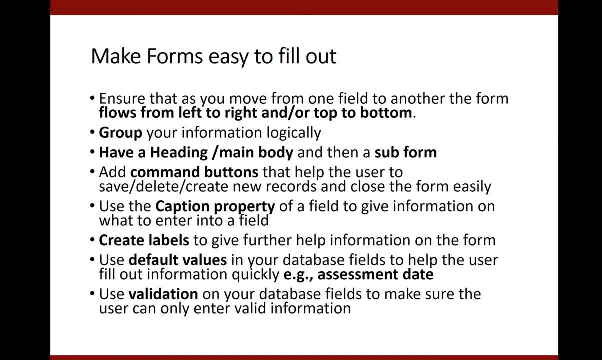 50 years back by going using the arrow. so I would just use the input mask and I would put a caption underneath it and then I will create labels. so the labels, they need to be spelled out, they- I will not use abbreviation for labels- and also you can use labels for extra information, for example for help, if you want to. 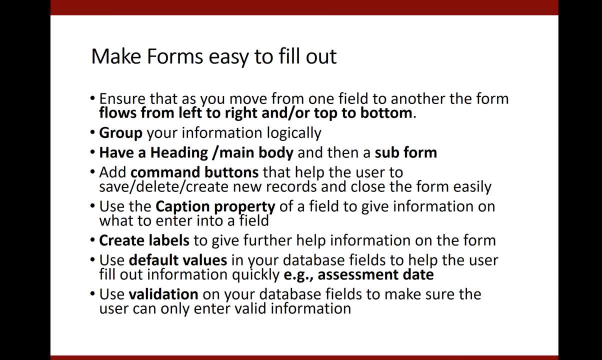 explain to the end-user what we mean here by history of falling, and then you can add more information or description of that and in another form so, and then you can put a label as kind of head for help, and then they can click on that help button and then 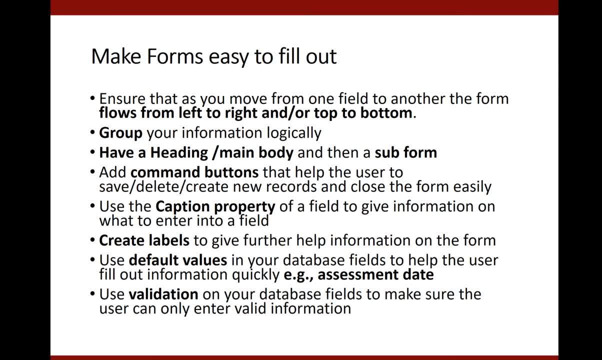 another window will come up with pop-up that has more details about the that particular field, for example- and I will show you an example, maybe in a little bit, what I mean by that- and then default values. remember when we said default values. for example, the assessment date needs to be defaulted to the now. 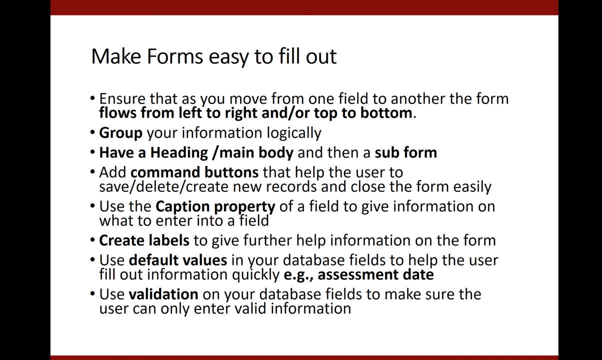 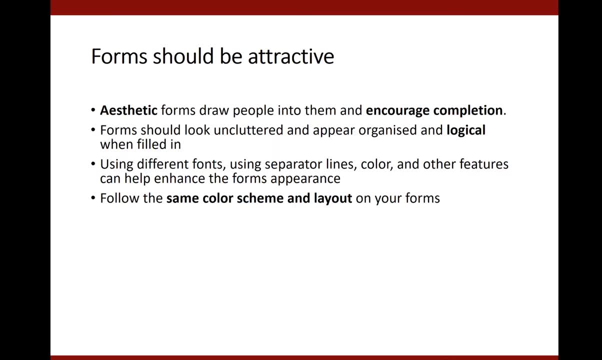 function where you show the date and the time that is current when that assessment was created, and then validation, if it is applicable. I would definitely use validation and we have done validation rules examples in class in the past. so aesthetic, and I can't emphasize it more: aesthetics or beautiful or attractiveness of the forms and reports. 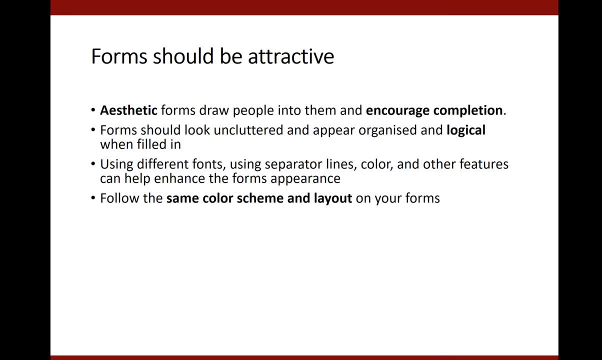 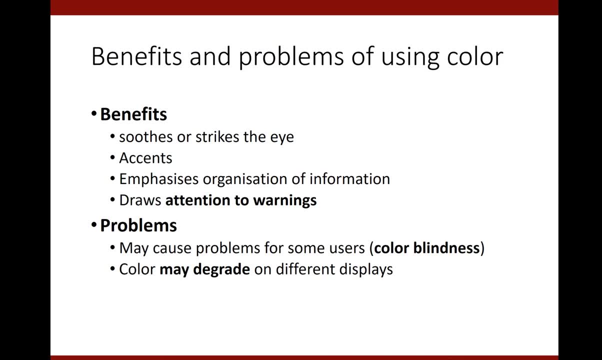 is is very important because it encourages completion, and so there are benefits and advantages and disadvantages of color. so we can. one of the advantages of color is that it soothes the eye, it emphasizes the organization of them for information, and it also helps us with attention to 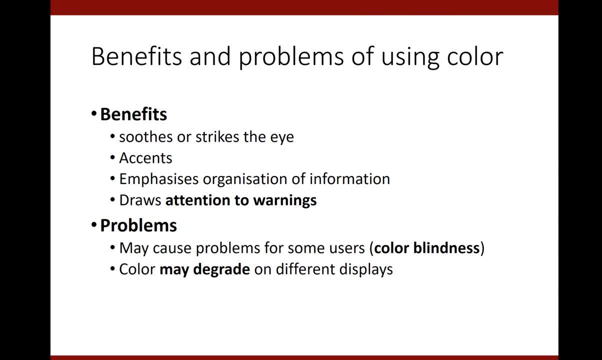 warnings. for example, if you are using a red color, that might be a warning and and one of the problems with colors is that there some end-users might be color blind, so we need to keep that in mind. and also, depending on the machine, you might see something as red, but when you open it in another machine or in the in the 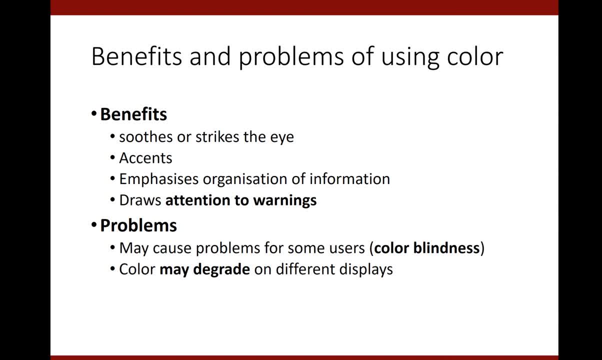 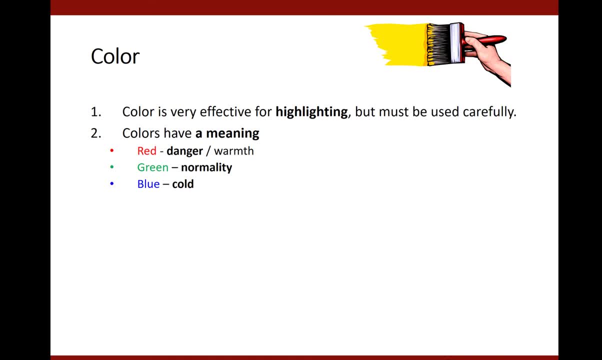 school computer that you are where you are presenting it might degrade the the quality of that color, so we need to keep that in mind. so color also can help us, highlighting some important information. and it also color has meaning. so red means danger, green normal. red means danger. and red means danger, green, normal. 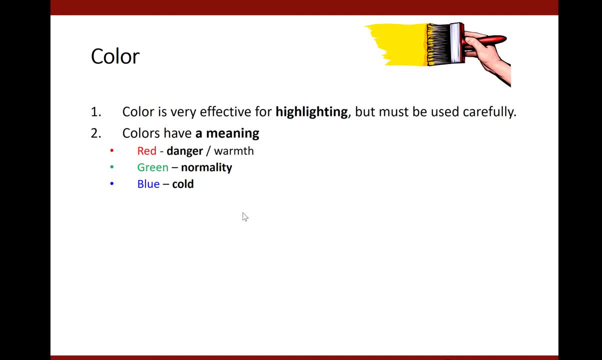 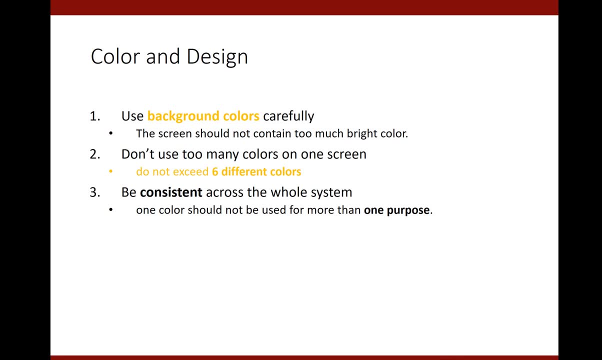 and blue is cold refers to cold, you know, and so on. so we it's important that we understand this about color. so color is very helpful, especially when we are using the background color. we need to use it carefully. remember when you did in tutorial 7- actually your case for tutorial 7- you learned how to use 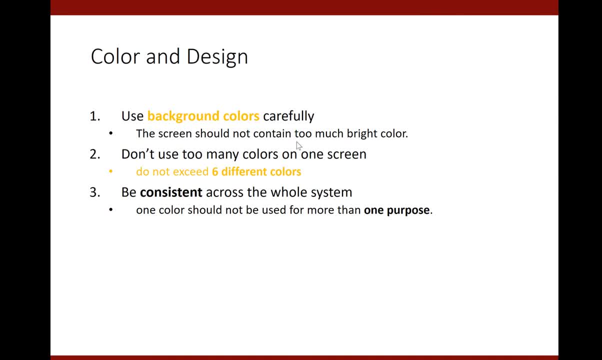 background color and how beautiful it looks when you are using the background color, so it can improve the attractiveness of your design, of your interface. so we will not. it is not recommended to use or more than six different colors. so I would not use more than six different colors, which is very. 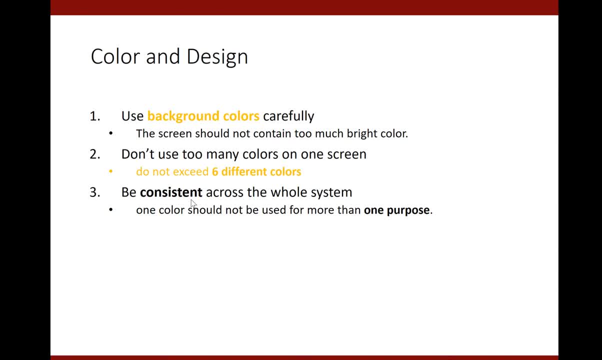 important. so and also be consistent across the whole system. what I mean here by consistent, as I mentioned earlier, so be consistent with the background color, for example, the title, the size of the title, for example, the color of the background color and so forth. so it's very important to understand. 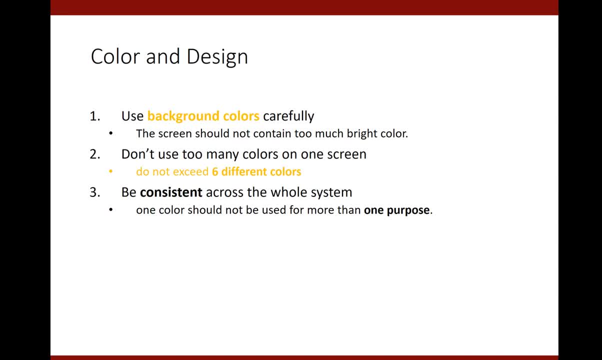 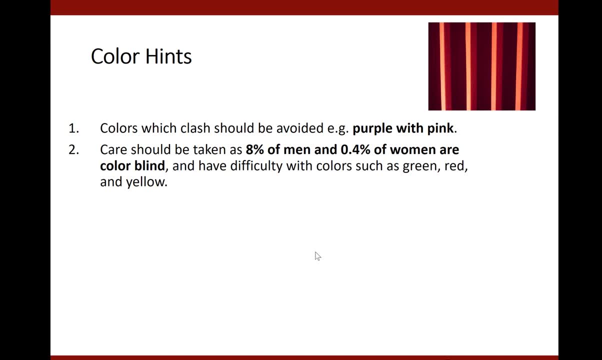 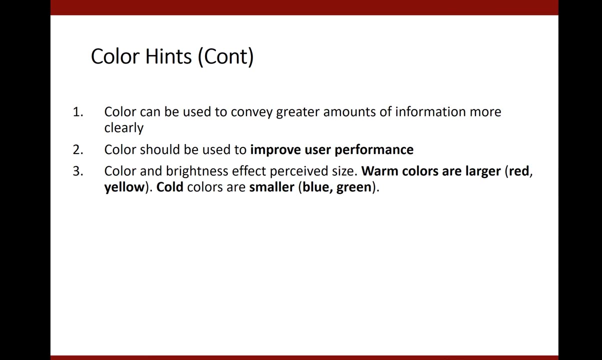 of the title needs to be consistent, the location of the navigation buttons should be consistent and so on. and also be careful with the overlapping colors. and also let's see another thing is for colors. we have warm colors versus cold colors, so the warm colors here include the red and yellow and the cold colors. 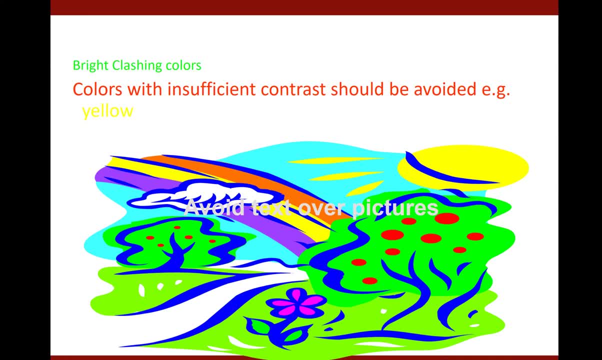 are the blue and green. so we will avoid using overlapping colors such as this ones, as you can see here. avoid text over pictures. you can barely see it. and the yellow over white- it, you can barely see this. this, this work. so we will try to avoid using some overlapping colors, so we will use more positive presentation. 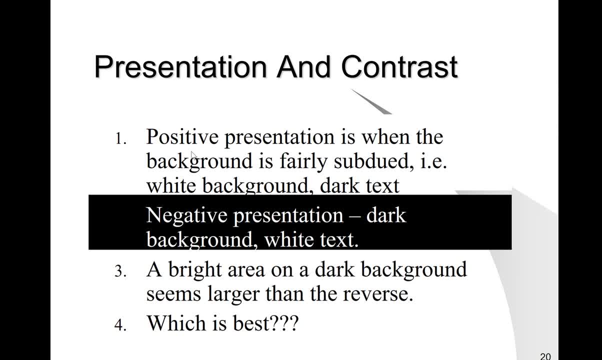 rather than those overlapping colors. so the positive presentation is what we mean by. that is an example, like when we have a white background and black text: in this case it is called positive presentation. so if we are using black background and pause and white text, in this case it is called negative presentation. so which, which one is best? 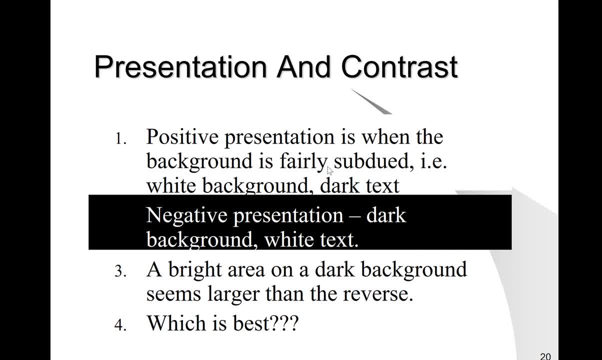 you can. you can actually, it's up to you, but I would avoid using black back background and white text, so I'll definitely use the first one, but it's up to you to do the decide for your own, but the most common rule. that's why you see, 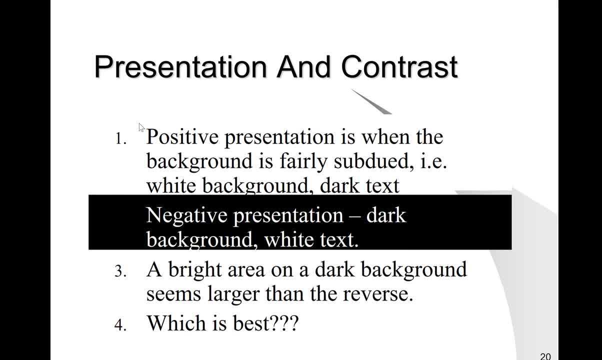 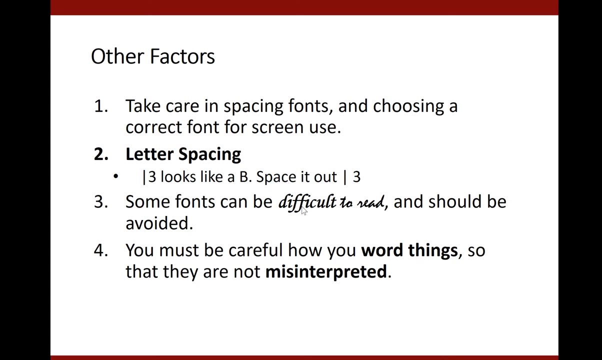 Google always uses white background and all other other companies are using white background or bright background, and if the negative presentation was was helpful, actually Google or Facebook and all other companies would have been using it. so again, that's kind of an indication that positive presentation is more powerful and much preferred, so we 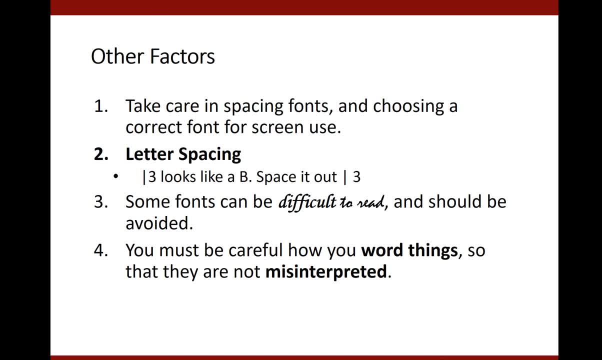 will need also to be careful when we are using letter spacing. as you can see here, space. if we don't have space between the dash or the, the mark, the hash mark or the, and also that, the three, it looks like it is a, B and so on, so we will need to not 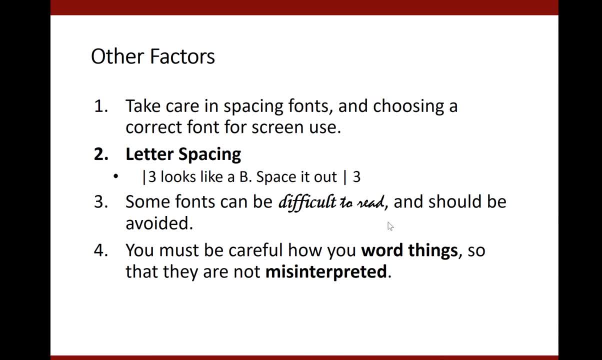 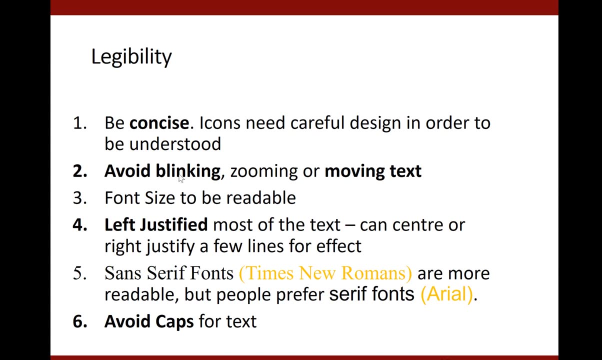 use hard fonts to read like this one, and also we will be careful with the wordings- how to word things- and have with misinterpretation lisibility. so we need to be concise and we need to use icons that are meaningful. for example, we can use like the: 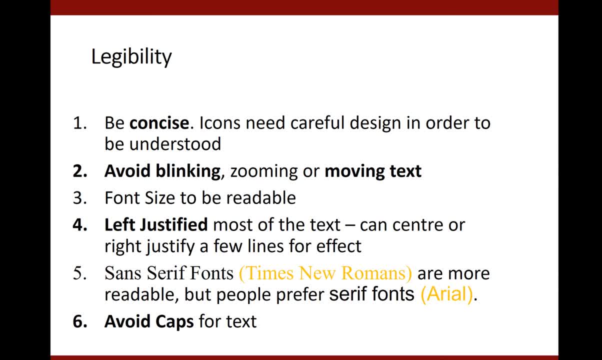 exclamation mark, for example, for questions or for. we can use, let's say, question mark for questions or we can use. so we need to be careful when we are using icons and then we need to avoid using blinking or moving text or because actually they are distracting the end user from doing the tasks that they are. 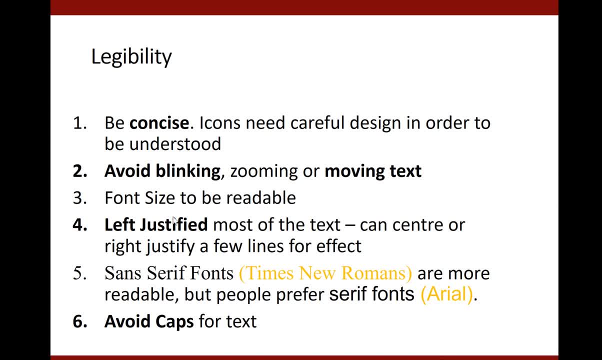 supposed to. and then we should always strive to left justify. in some cases you might, but we will definitely try to always left justify. and then there are two types of, two major types of fonts. there is the sans serif fonts, which actually has edges in there. they have sign of nodes or in their 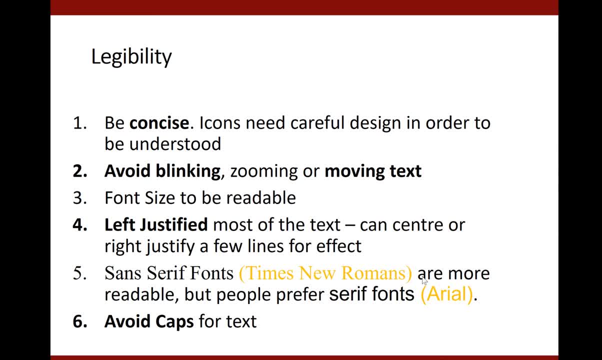 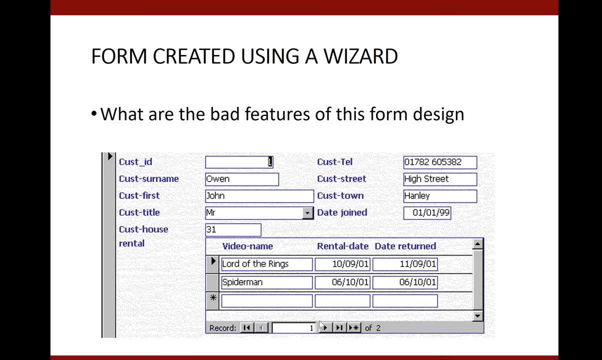 edges, such as Times New Romans. as you can see, they are more readable, but most people actually prefer the serif fonts, which is Arial doesn't have any nodes in their edges, so we'll try to average caps for text as much as possible, so I want you to look at this one and try to identify them. 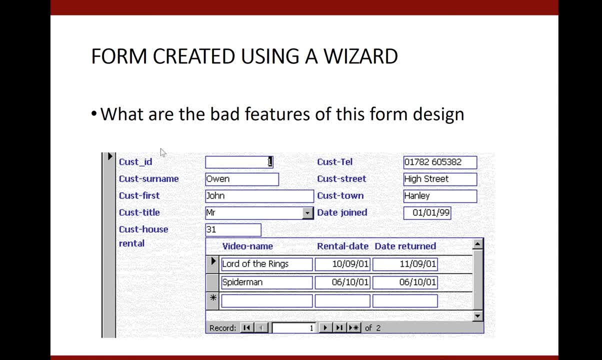 pause for a moment and try to identify what is wrong with this for so, so I'll let you think about it now. there are a couple of things that are wrong with it. there is no logical logical the labels: they are not spelled out. there is no. this customer ID is not left justified. and also the the order, if you. 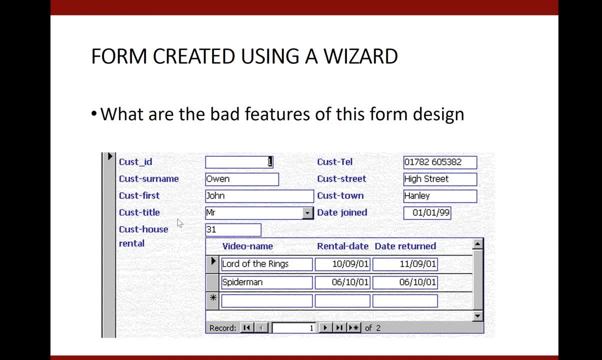 notice here we start with the surname and then first name and then customer title. I would start with the customer title, so it's not logical order. and then customer house is here and then moves on to the, to the, the telephone, and then the street. so the address is not grouped. so they need to be grouped, like everything. 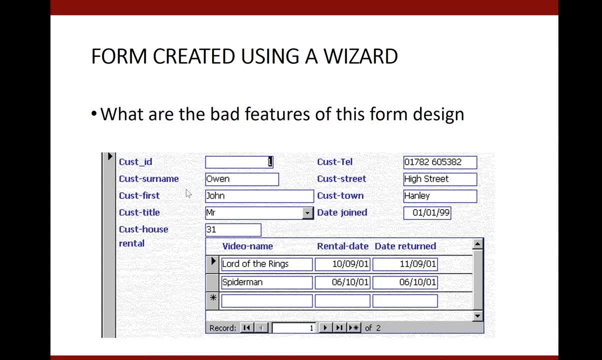 in one group by itself, and then I need to spell out the labels. I need to use color, I need. I need to have a meaningful title for each of those groups, or a title for the form and the title for the each group. I need also to have navigation buttons, and I don't have them. 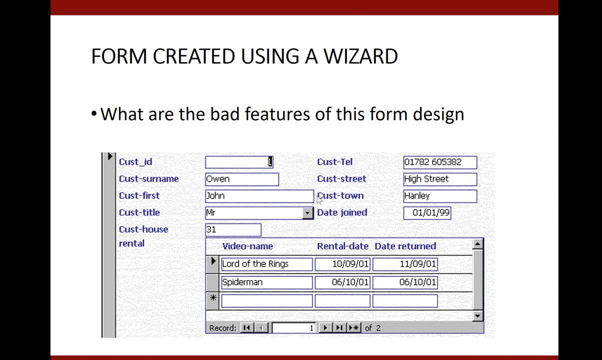 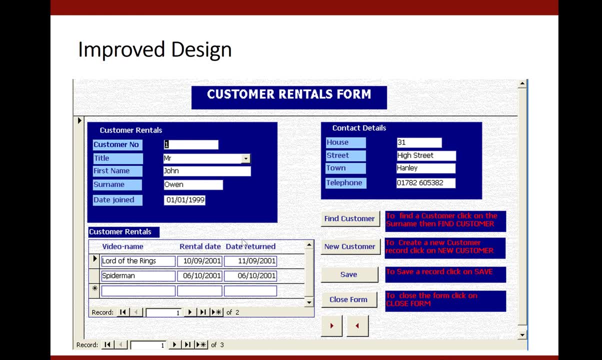 I would never use those navigation buttons that are here. I need more meaningful information. so this is a much better one. it's a little bit more improved. so there is, there is a title, there is really efficient use of the colors here and there and they have buttons and they. 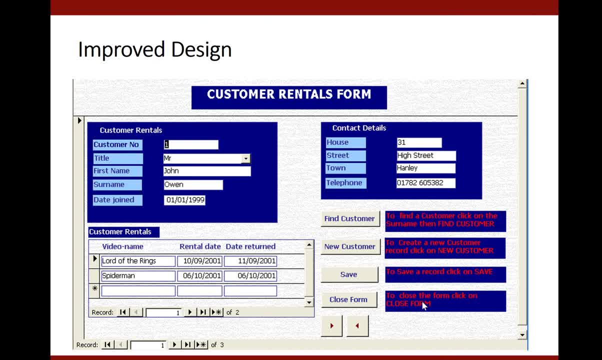 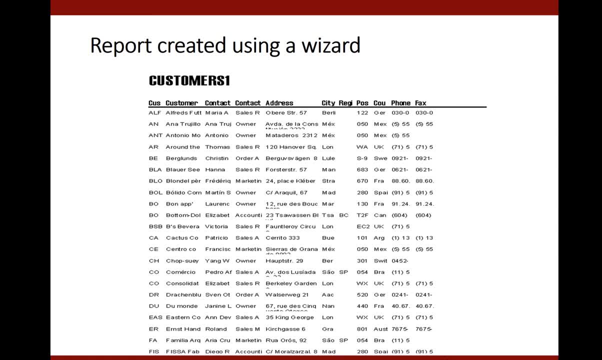 have labels or captions explaining what each one of those buttons do. so you get the idea here. so this is another battery design of a report. so it is all listed in one page and, as you can see, some of these is missing. for example, the addresses have cut and it's not, and also the titles. they are not spelled out and 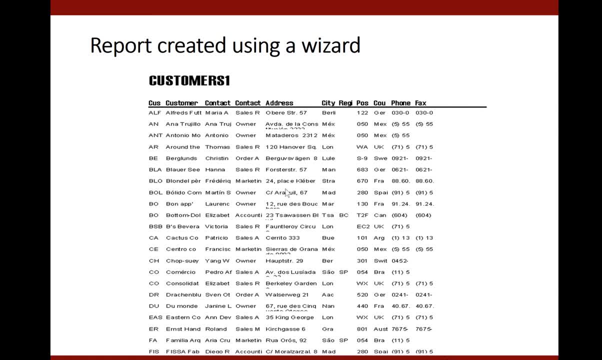 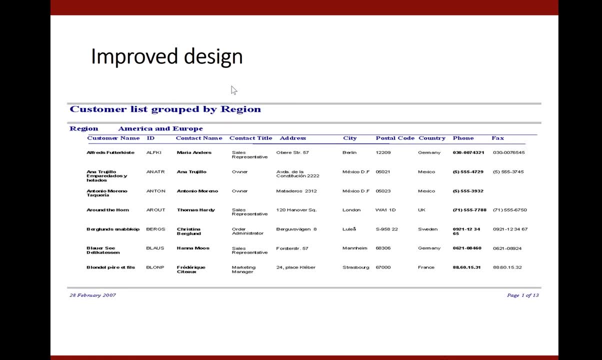 they are not clear. so this an example of a bad design for the report. so now, and also the title of the report is customers one. it doesn't make sense. but here we have customers list grouped by region. it's more meaningful. and then they are grouped by and they have lines that we learned how to use them and they have. 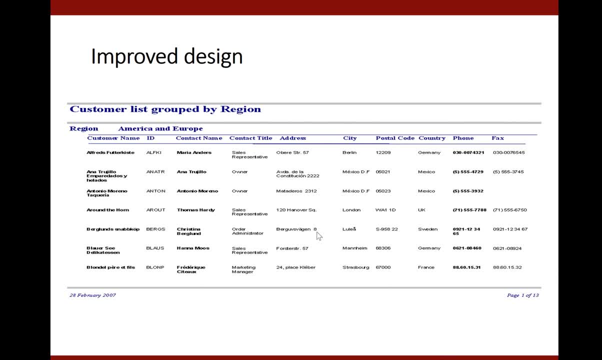 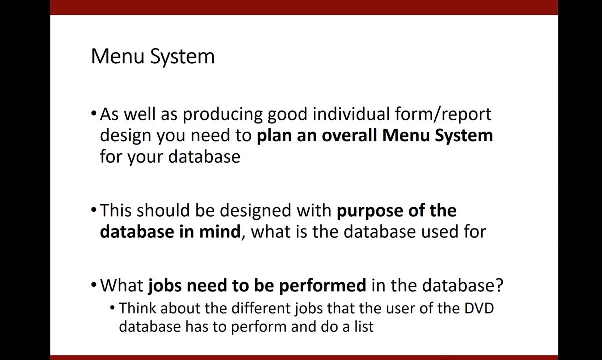 highlights and they have bolds and they have it, so it looks much more beautiful here. so again, it's very important that we have a menu system. so the menu system is very important because it helps us kind of to to plan where we start and where we go from there. so, depending, 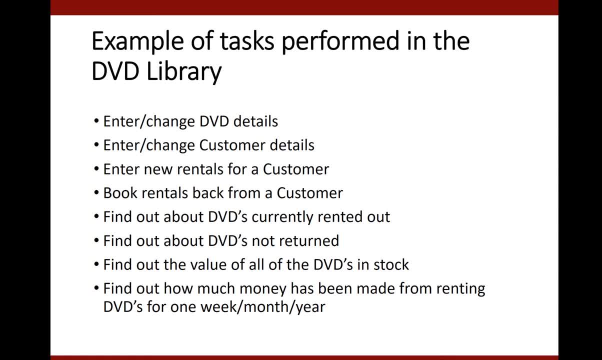 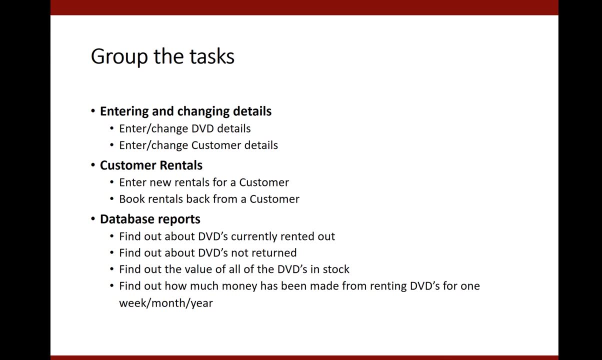 on the purpose. you can identify all the tasks that you want your end user to go through or your system to perform. then, based on those tasks, you can put them into themes, and then every theme uh, is you know, is it is in a group, basically, and then you can create buttons. 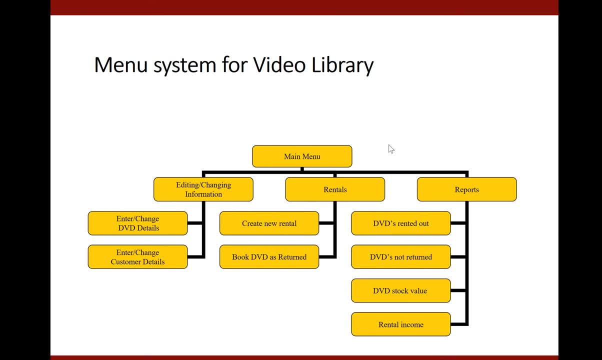 for them. so this is kind of an example of a hierarchy or a menu system. so the menu system- uh, in our case we will have reports is one of the branches, and then we have four reports and you can double check with the request for proposal. what are those reports? 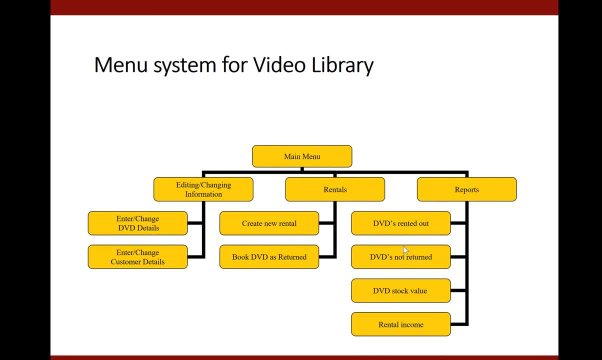 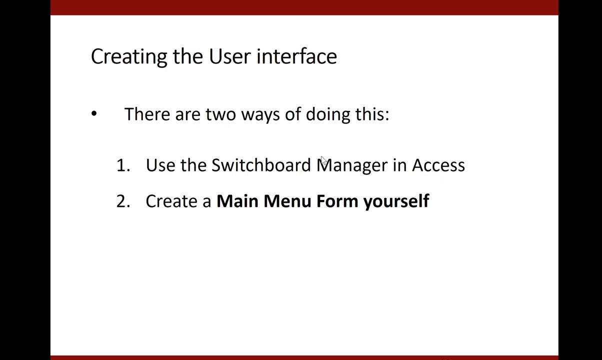 and other documents as well, show what the reports are in details and then forms in in our. in our case, we have only two forms that we are interested in for the end user to be able to access is the resident form and the assessment form. so that's all that we want for the main menu. so the main menu, that's when the the default. 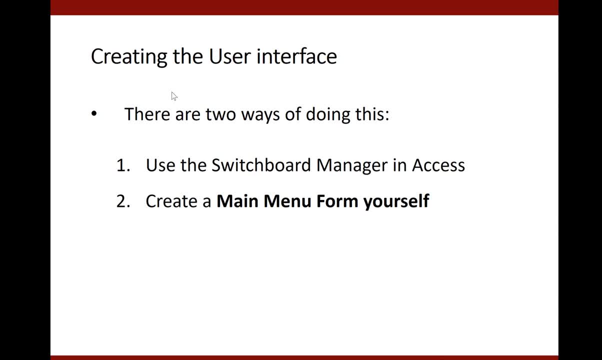 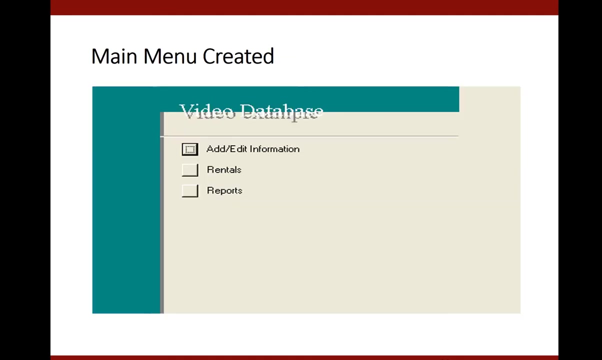 form that the end user gets into. so creating the user interface so you can create a navigation form or a main menu form using switchboard, so switchboard manager in access. and another option is to create your own main menu using and down form. so this is an example of switchboard which i 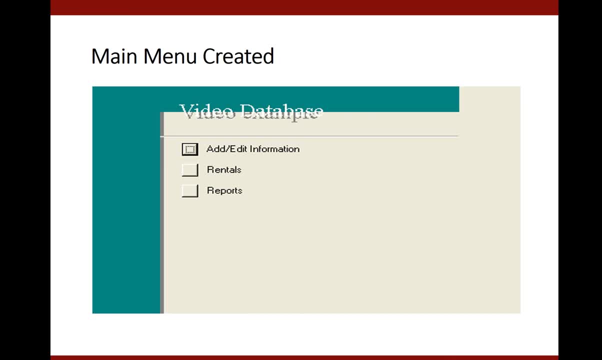 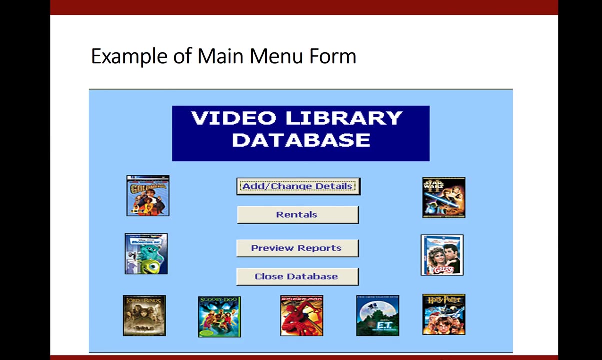 actually personally don't like the switchboard that is generated by microsoft access, because it doesn't look professional and it doesn't give you an option to do more to it. uh, it is very limited, so this is based on a form that you yourself can create and bound form, so blank form, and then create the buttons, add the buttons, add the colors and 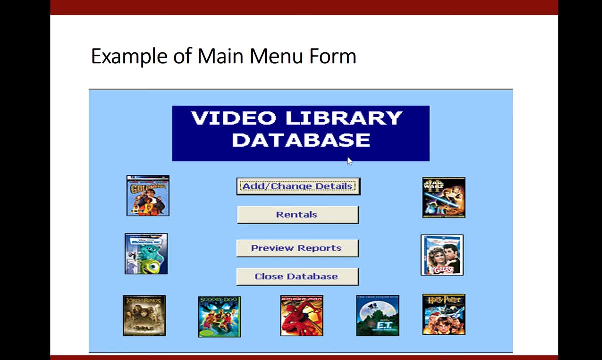 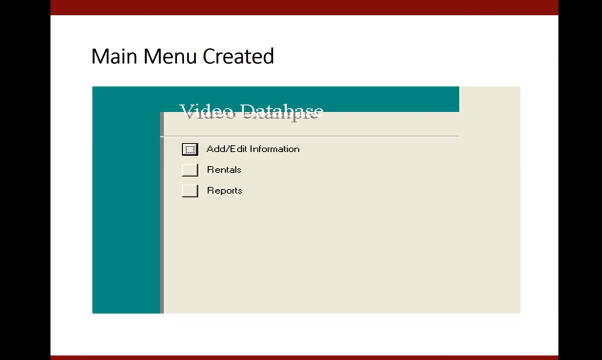 pictures to it, and so on. so this is much more beautiful form than the switchboard, which is very dull. so this is what i would recommend: create something that you yourself design, rather than having- uh, you know- the switchboard dictate to you what to do. so, again, this is a summary of what we have done. 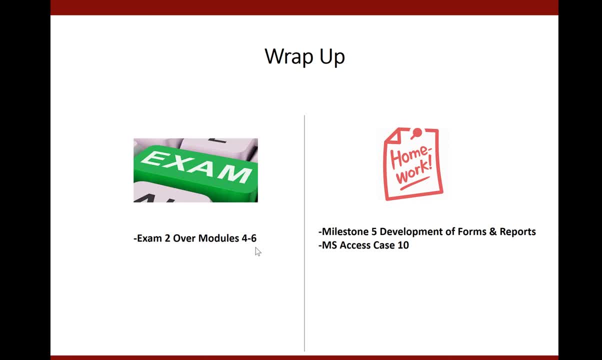 and remember that we will have exam two over modules four to six, and so we are going to emphasize the content that we have talked about in class, including the sql statements- retrieving data from one table and retrieving data from multiple tables- and also we will emphasize the content that we talked about since 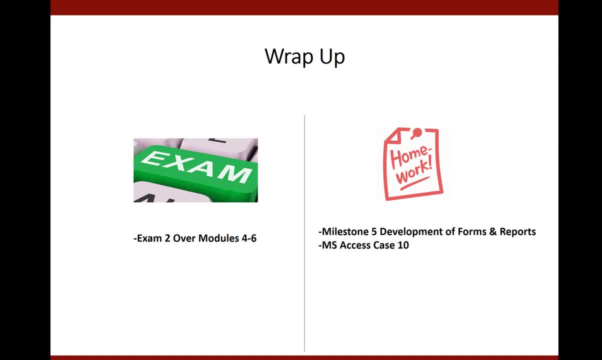 so we we talked about where to put the foreign key, for example, the rules of thumb. those are some of the questions that would be asked. and then normalization process: we talked about it, so that would be covered in the exam. so it's going to be multiple choice. it's going to be